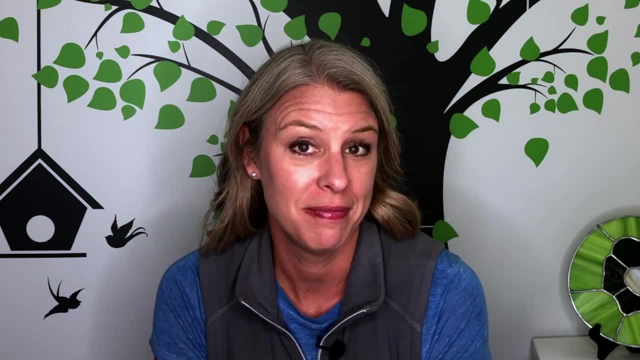 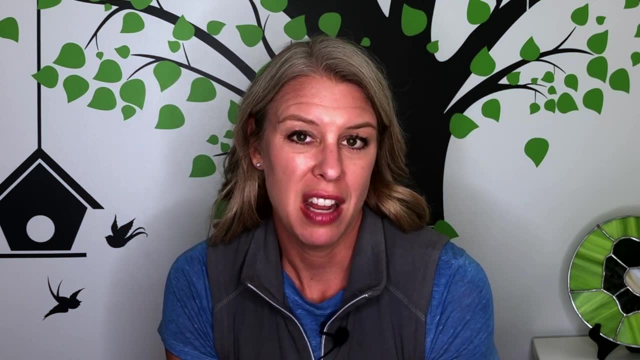 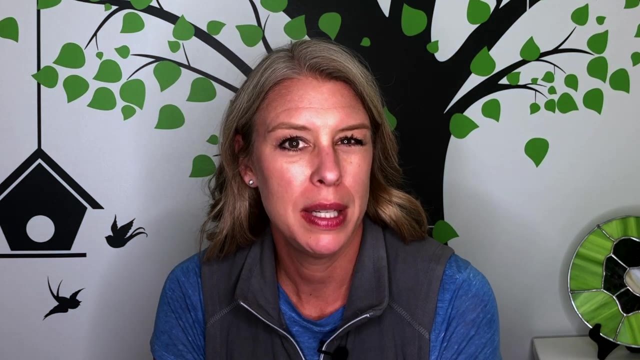 be last if I made some adjustments to my training and to my eating. The first thing I discovered was, even though I wasn't overweight, I wasn't necessarily thin. I lost a few pounds. My times got faster. Next thing I realized was drinking water makes a big difference in fatigue. I started 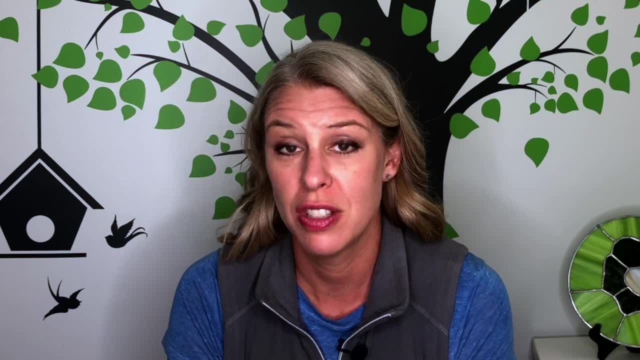 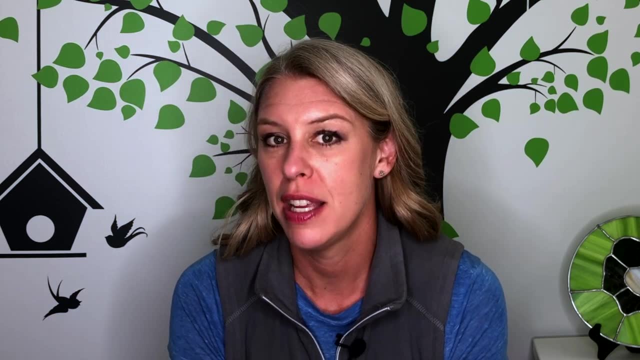 drinking before I exercised, drinking during exercise and I started drinking some water. I confuse water after exercise and found that my endurance was much better. I continued to learn about sports and nutrition, about carbohydrates and protein. Every new thing I learned improved my performance. 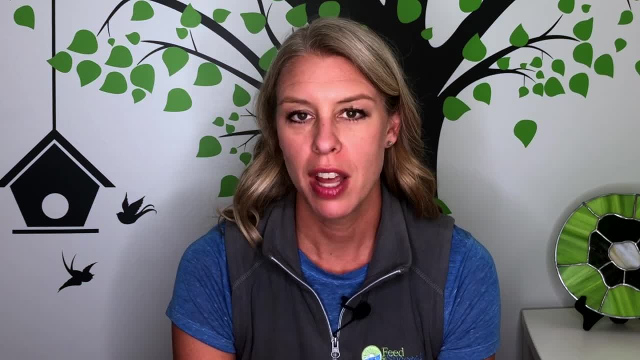 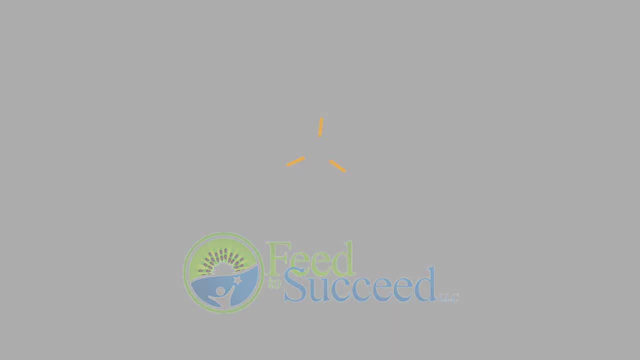 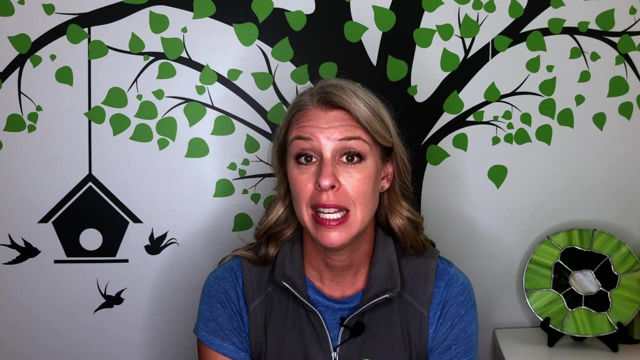 I'm Betsy Jelmgren with Feed to Succeed. Today we're talking about sports nutrition. When kids get into middle school or high school, the demands of their sport start to increase. The more serious they get at sports, the more they take up physical activity. 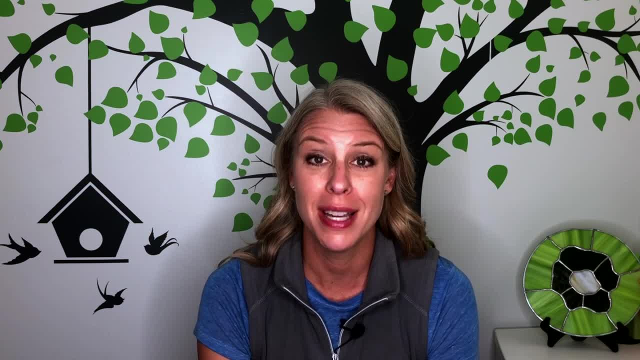 The more serious they get at sports, the more serious it gets at physical activity. The more serious they get at sports, the more serious they get at physical activity about their sport, the more diet can have an impact on their performance. When I see kids and teen athletes who have dietary restrictions, sports nutrition gets. 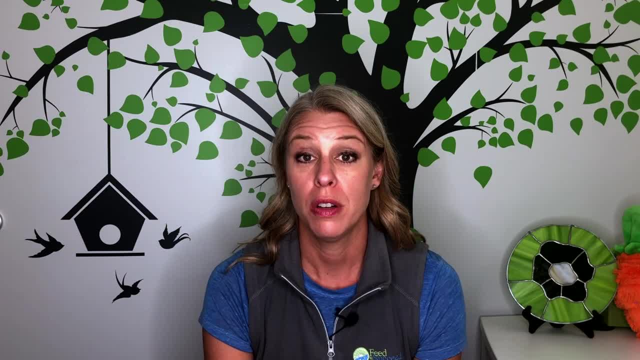 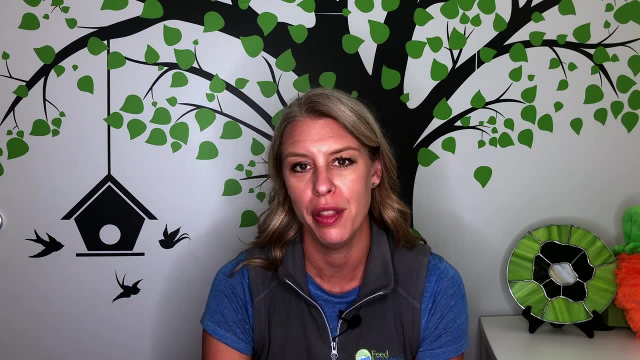 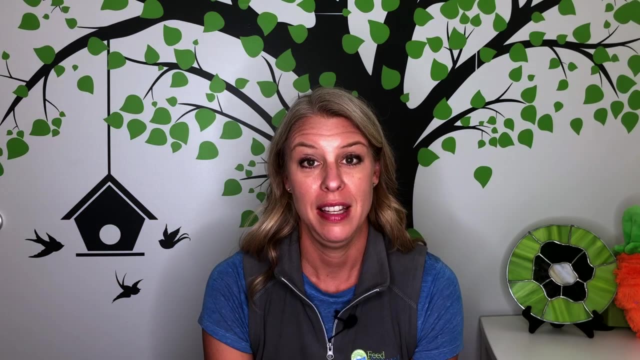 more complicated. Today, we're going to talk a little bit about what you can do to help your kids and your teens, who are athletes, to get the nutrition they need, both for performance, but also for optimal health and growth. Diet influences everything for an athlete, from illness and injury prevention to building. 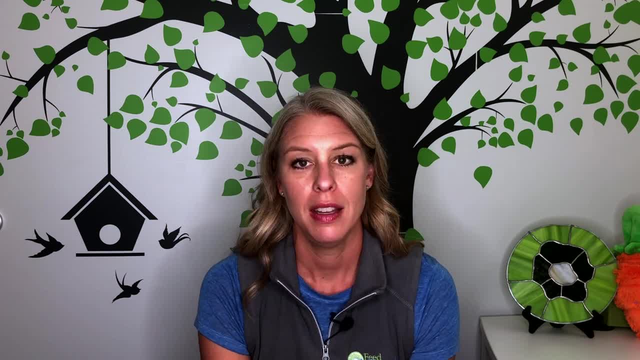 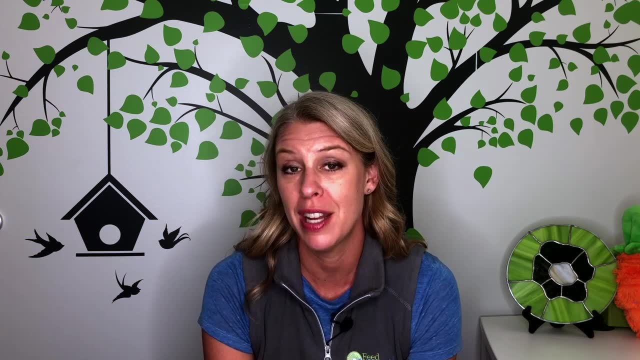 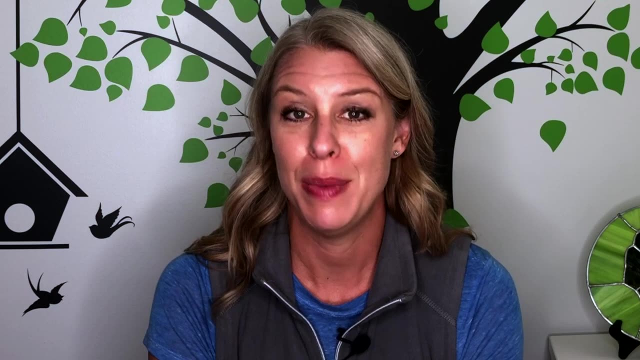 strength and endurance. There's a lot that goes into it. In fact, nutrition has such a big impact on athletes that most professionals and Olympians work directly with the dietitian to figure out how to eat to maximize their performance. Becoming a well-trained athlete is probably the ultimate in becoming a healthy eater. 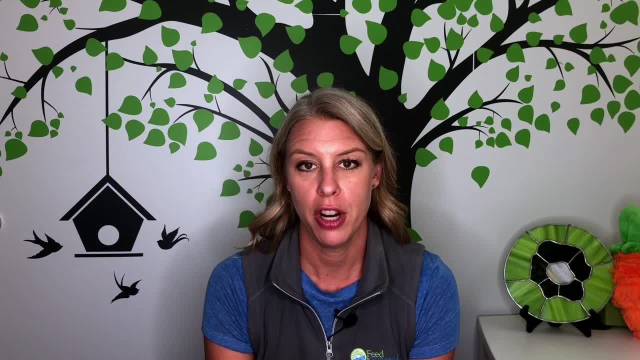 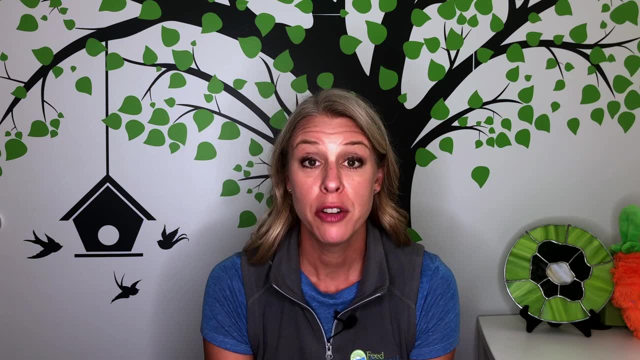 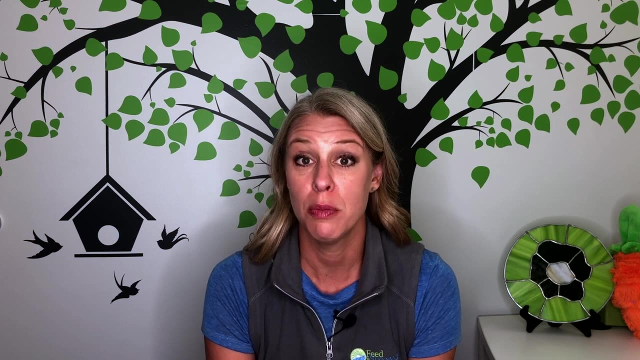 Let's take a look at what dedicated athletes need to stay at the top of their game. 1. Complex carbs- Carbohydrate- is a rich source of energy for brain and muscle tissue. Athletes use a lot of energy, especially in their muscles. They need extra carbohydrates before they exercise to fill their muscle stores, they need carbohydrates during exercise to keep them going and they need carbohydrates after they exercise to replenish the used-up stores. Most athletes get complex carbohydrates from whole grains, Whole wheat breads, whole wheat bagels and things like that. 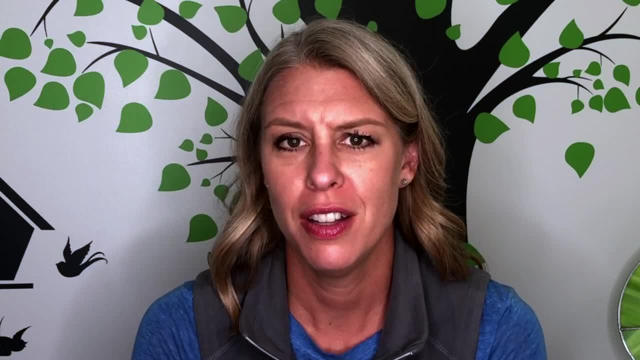 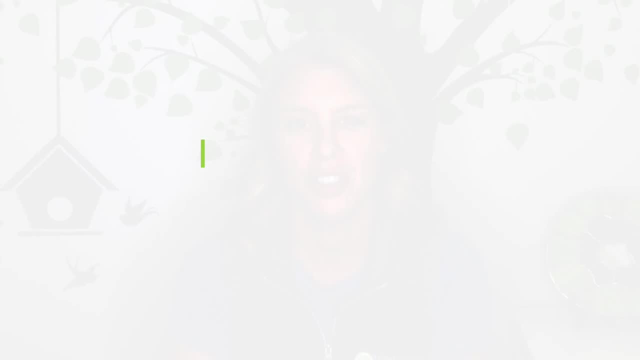 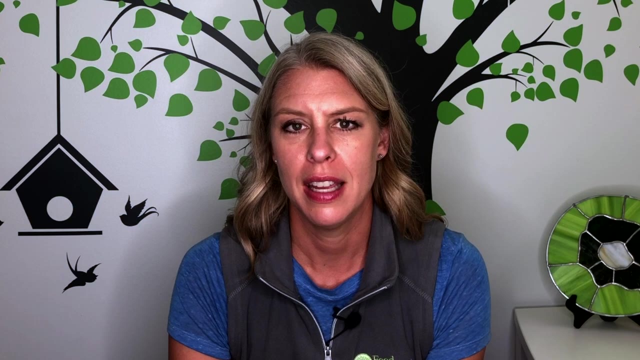 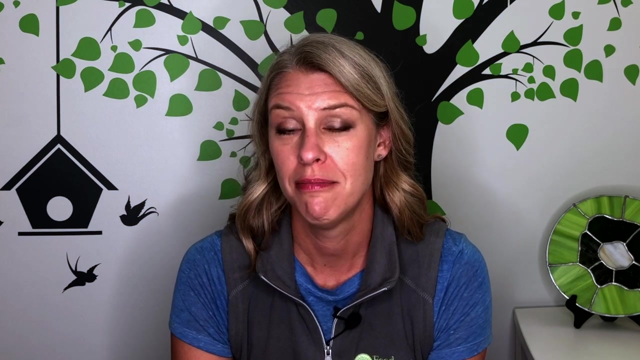 Other sources of complex carbs include potatoes, cereal, pasta and rice, to name a few. Protein is also essential for athletes in order to build muscle and help repair tissue. Protein sources include animal proteins like meat, chicken, fish, eggs. Also includes dairy products, milk, yogurt and cheese. 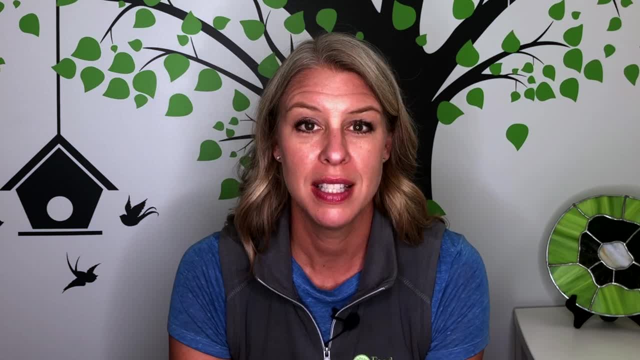 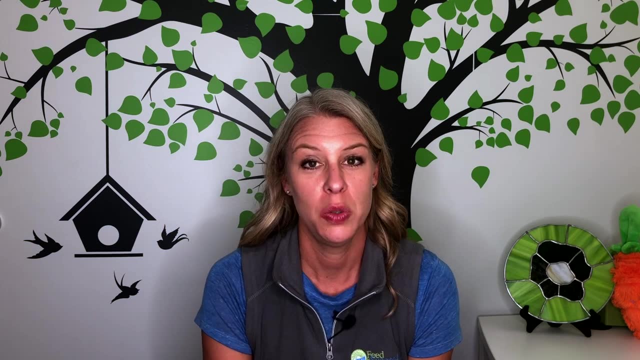 And plant proteins like nuts, legumes, even some vegetables like spinach. Athletes need other things too. They need to be hydrated, such as water. They need electrolytes, which is salt, but it can come in the form of supplements or 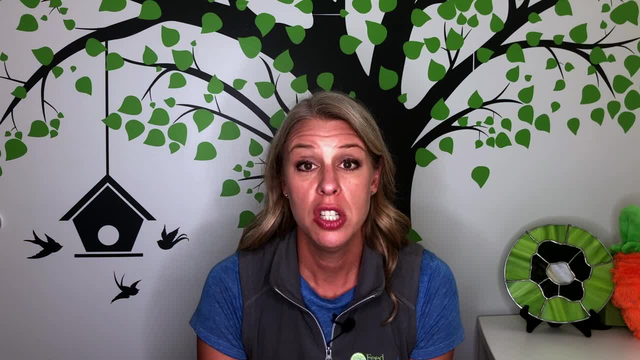 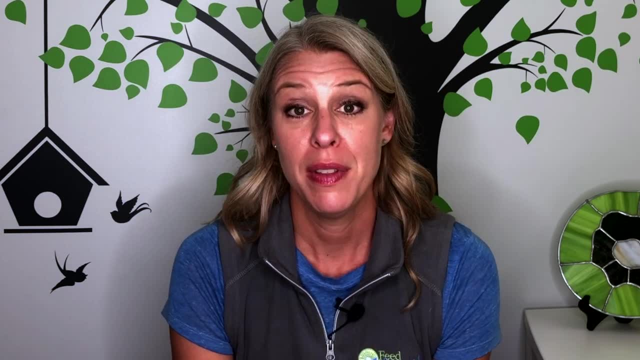 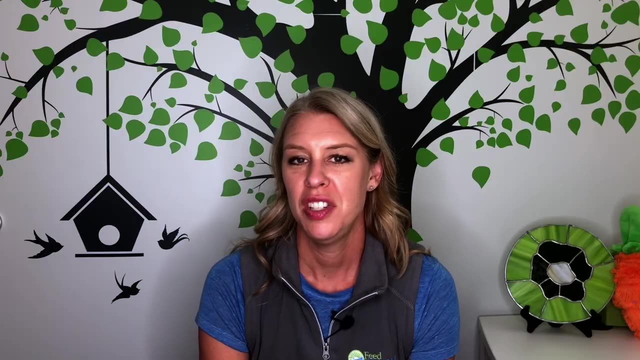 other foods. Athletes need fruits and vegetables for tissue repair and healing and injury prevention, And additionally, there's lots of supplements on the market. Some of them are good, some of them are bad, but those are things that athletes may be using and navigating as well to contribute to their training program. 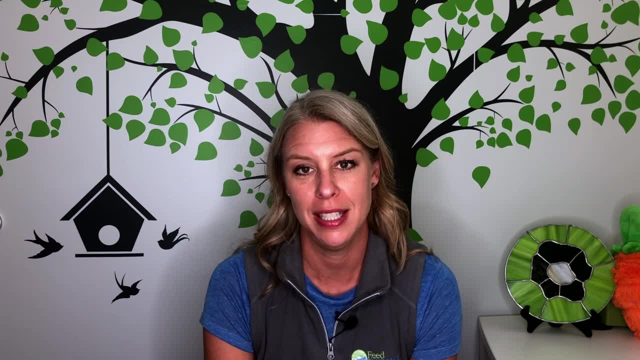 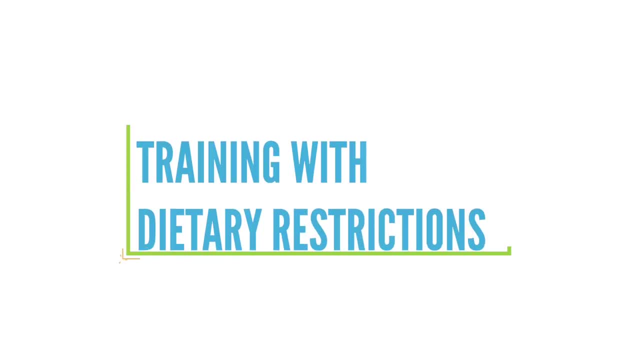 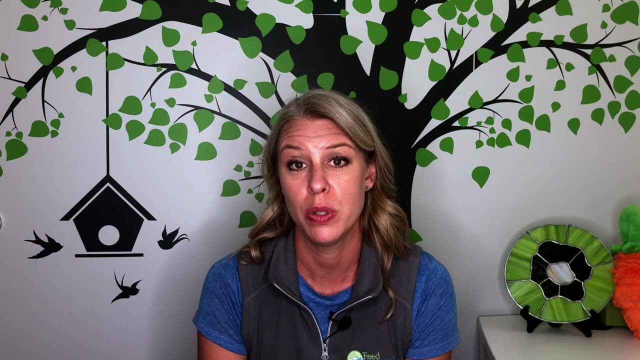 As you can see, athletes have specific and demanding nutritional needs, But people with dietary challenges can't always meet these needs in traditional ways. In my practice, I work with many kids and teenagers who have specific diagnoses, So then we're looking at other dietary factors that need to be put into place to help the child or the teenager get well, Okay. So if you have specific needs of an athlete on top of that, it can get really complicated. Some of the more common things I see in my office are athletes who are underweight or athletes who have IBS. 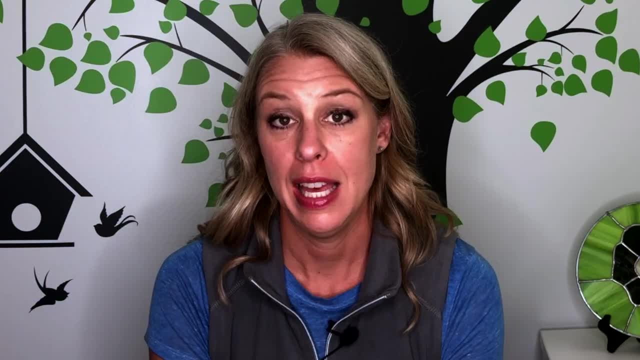 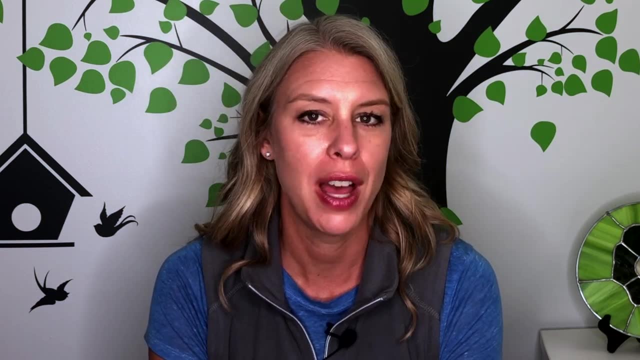 Another thing I often see is gluten intolerance and celiac disease. Athletes who have celiac disease or gluten intolerance are cutting gluten out of their diet, which eliminates a lot of our options for complex carbohydrate foods. Additionally, when we eliminate some of those foods, we're also eliminating some of the 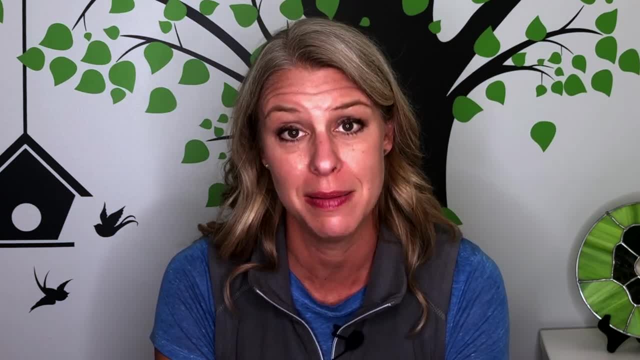 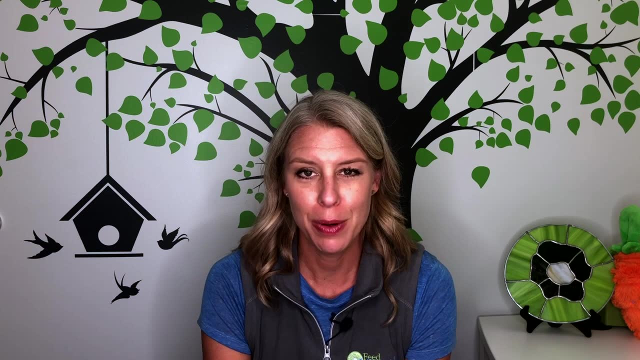 nutrients that would naturally be there, such as some of the B vitamins. B vitamins are essential for energy metabolism and a number of other bodily functions. They can be replaced and athletes on a gluten-free diet can do great, But sometimes they need some guidance. 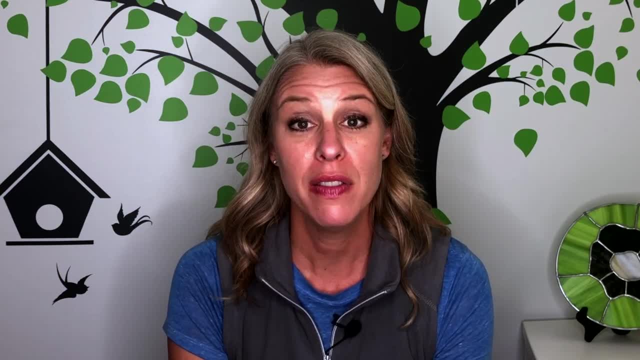 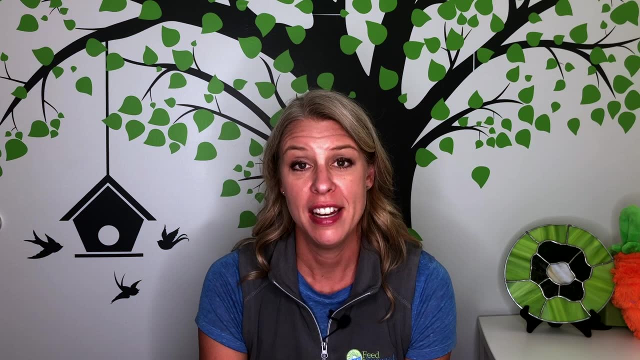 While there are many gluten-free food options on the market, many of them are pretty refined, not as much whole grains and whole food. Additionally, people on a gluten-free diet or on any kind of diet restriction have to be very careful about reading labels. 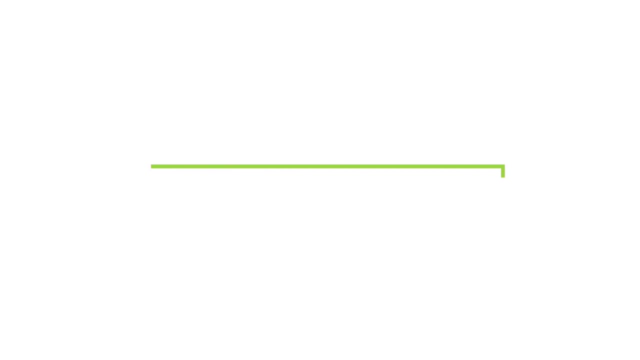 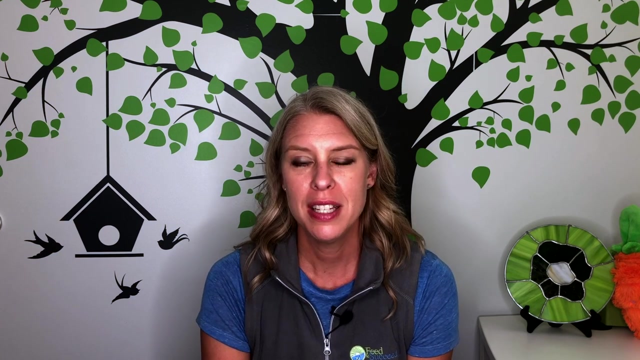 And if they don't have any of those, they're likely to be underweight. A dairy allergy would be hard for me personally as an athlete, because I use so many dairy products for post-workout fuels, like yogurts, chocolate, milk and cheese. Dairy products provide athletes not only with protein and carbs, but with calcium. Calcium is very important for bone mineralization and athletes can be at increased risk for stress fractures. It's important to address calcium needs And make sure calcium is being replaced on a dairy-free diet. For my patient athletes with IBS, we're looking to control a lot of things. Sometimes their symptoms are interfering with their practicing. We also may be doing dietary modifications to help control symptoms, such as in the case of when we put an athlete with IBS on a low FODMAPs diet. 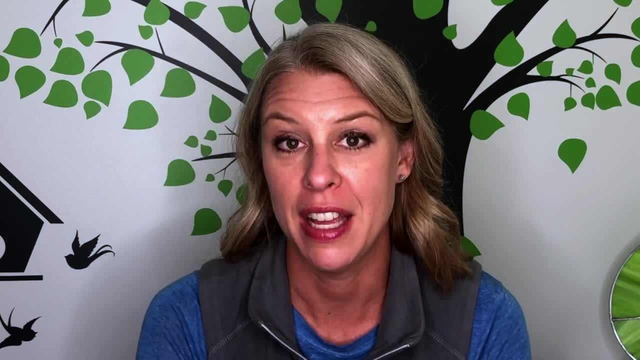 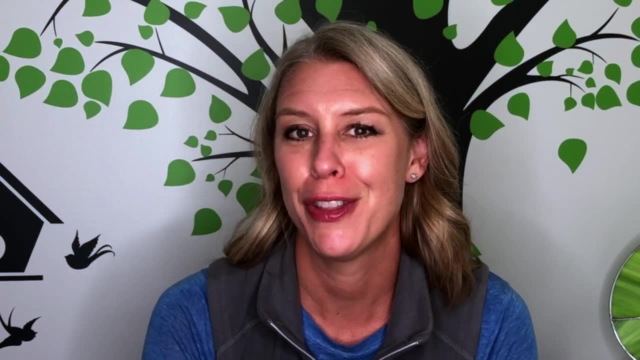 For my underweight athletes. often they're not getting enough calories in. This is leaving them in an energy-intensive state, And that's why I'm trying to control a lot of things. They need to learn how to make sure they're getting enough calories for their sport. 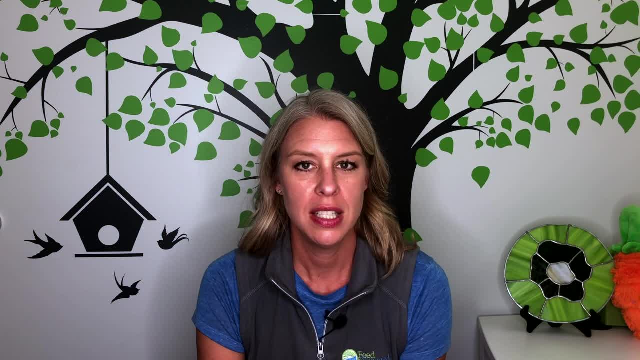 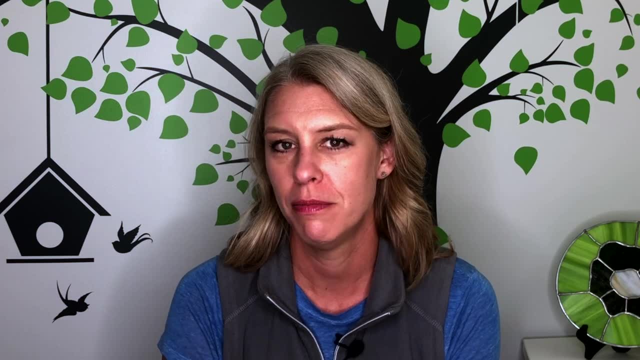 This all may seem very complicated, but with a little education and support all young athletes can thrive. Take, for example, the high school cross-country runner I worked with last fall Spring of sophomore year. she was doing great, having great times on the track. 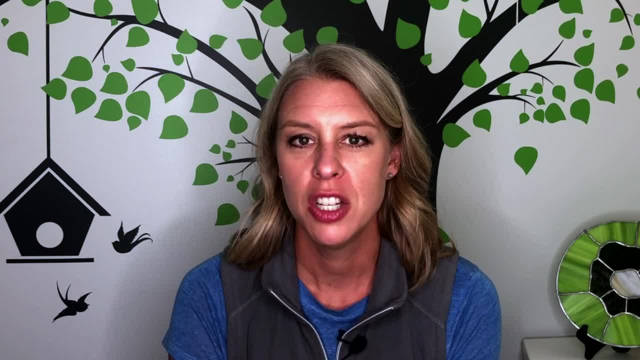 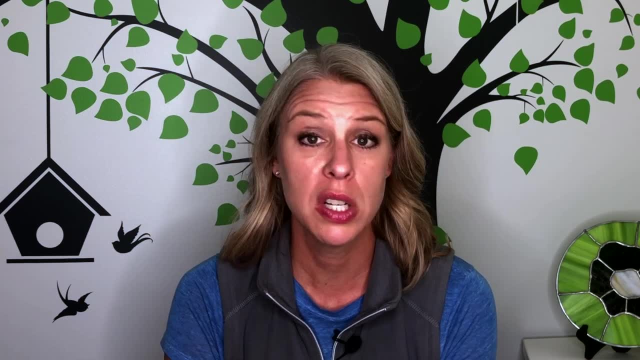 But when fall came around, something was going on with her health. She kept getting light-headed, Her times were slow. She was collapsing at the end of races. After meeting with her doctor and a specialist, she was diagnosed with celiac disease. 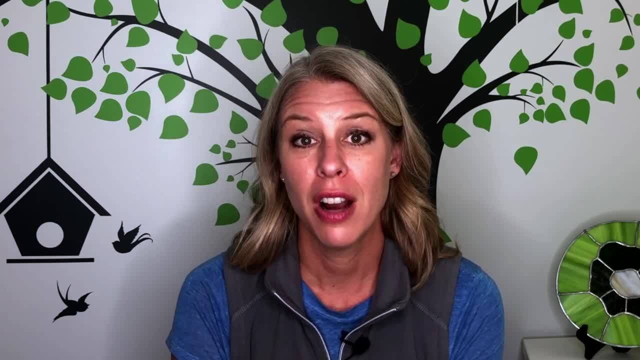 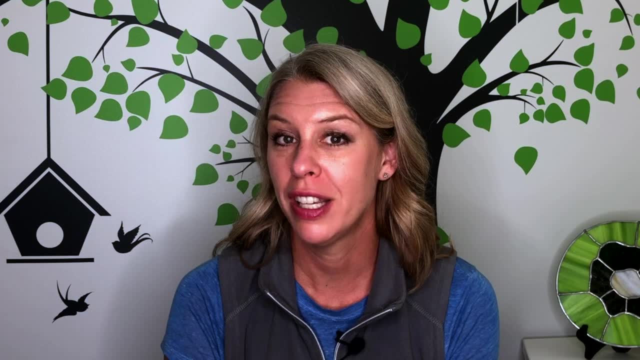 She hadn't been absorbing nutrition well. Her weight was down, her iron stores were low and all of this was causing difficulty with her ability to run. When we first met, we were focused on getting her on a gluten-free diet so she could start. 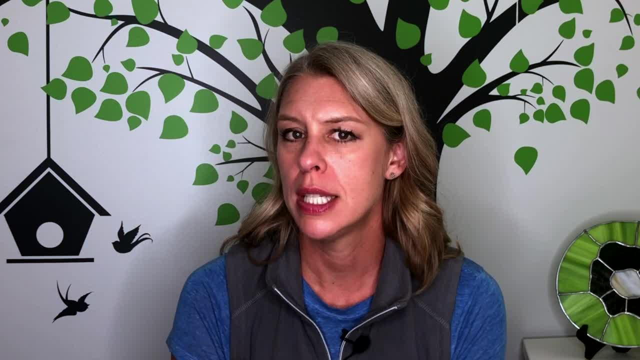 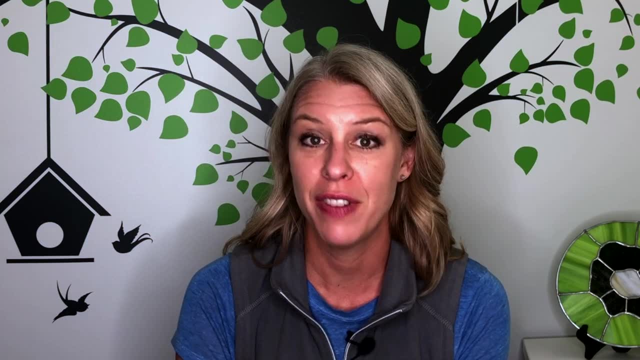 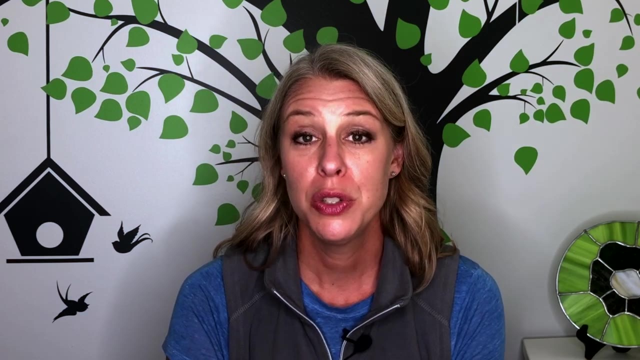 to recover, But in subsequent visits we started focusing on sports nutrition and replacing vitamins, protein and other things that were going to help her get strong again and get fast. After a few months of good nutrition, vitamins, protein and a gluten-free diet, she was strong. 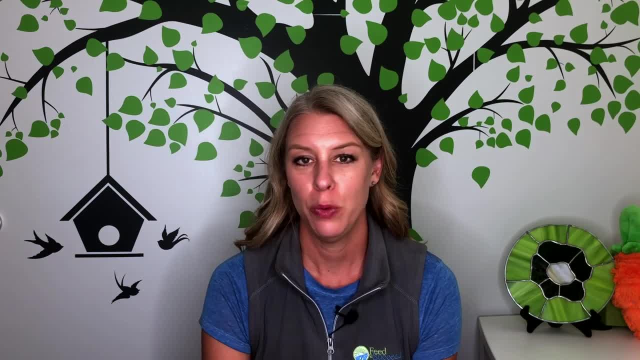 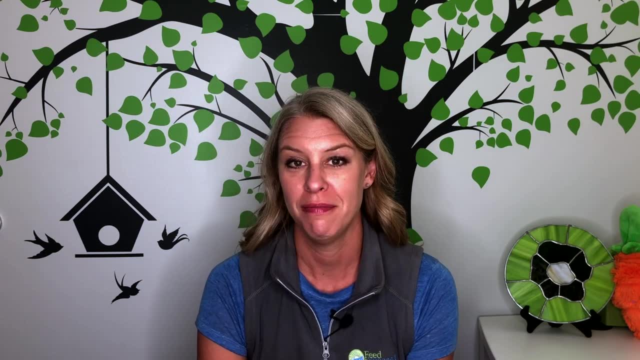 and her times were back on track. On the Feed to Succeed website, you can search for sports nutrition. You'll find blogs, articles and podcasts that will help you get more information. If you're interested in teen sports nutrition, check out our podcast with Alyssa Yelperin. 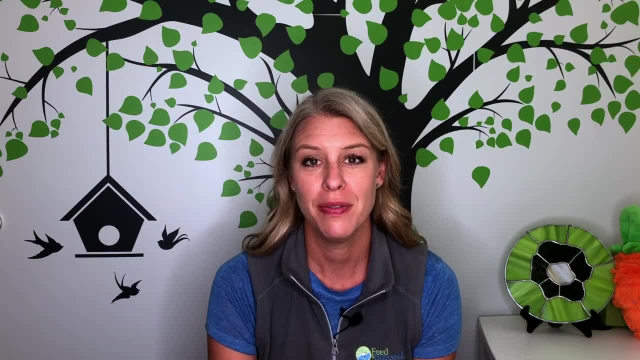